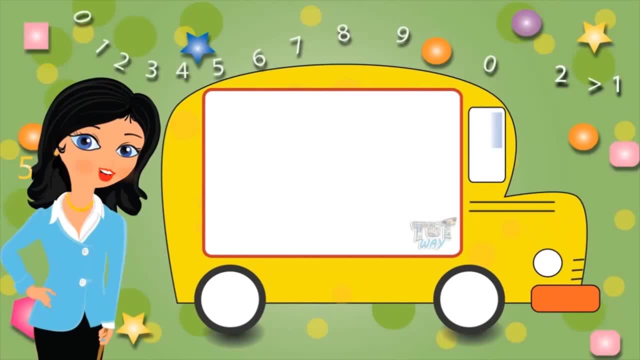 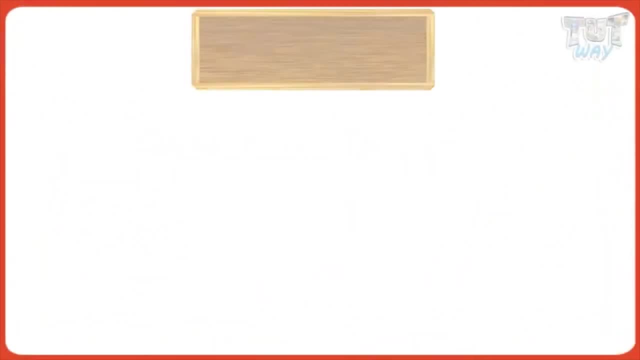 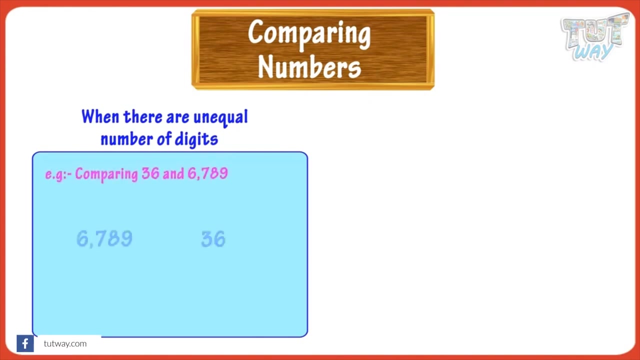 Hi kids, Today we will learn comparing and ordering numbers up to millions. Let's first learn how to compare two numbers. There are always two cases in comparing numbers When the number of digits in two numbers are different. rule of thumb is that the number with more number of digits is bigger than. 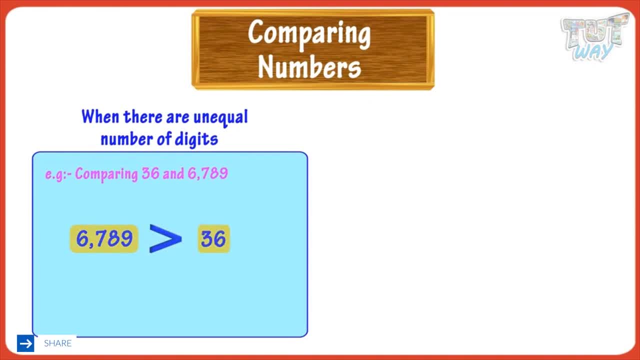 the number with lesser number of digits, 23 is less than 678, as 23 is two digit number and 678 is a three digit number. Here is another example. Here we have two numbers Digits. in both the numbers are different. 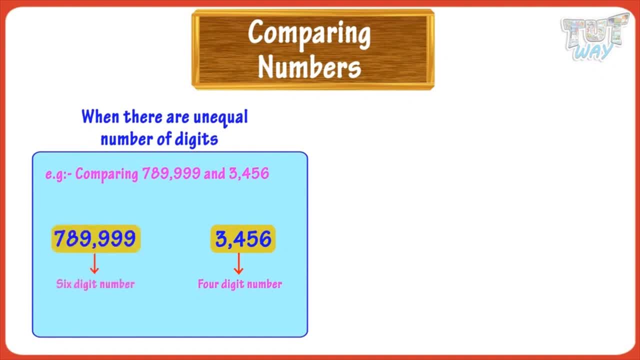 This is four digit number And this is six digit number, So we need not compare the numbers. Simply, the number with more number of digits is bigger. Second case is when the number of digits in two numbers is same. Let's learn how we compare numbers when the number of digits in two numbers is same. 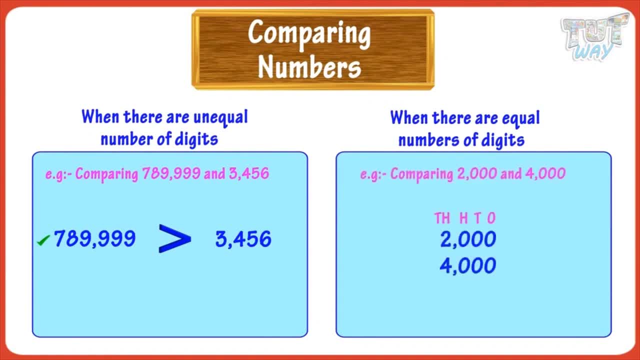 First we compare the numerals at the biggest place In the numbers. So we will compare the thousands place here. Four is bigger than two, So the number with bigger numeral at the biggest place is bigger. So four thousand is bigger than two thousand. Let's take another example. 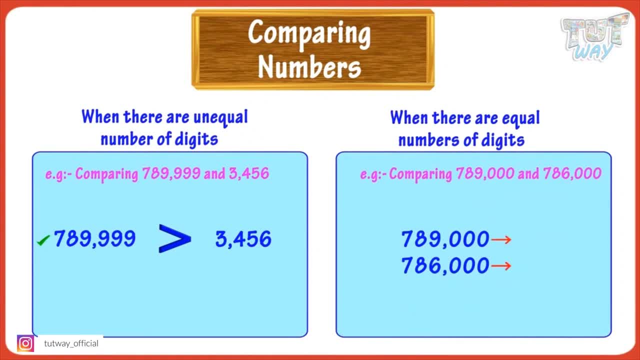 Here too the numbers have equal number of digits. Both have six digits. First we compare the digits at the biggest place. Both are same. So compare the next digits Again. both are same, So move. the next digit, Nine, is bigger than six. 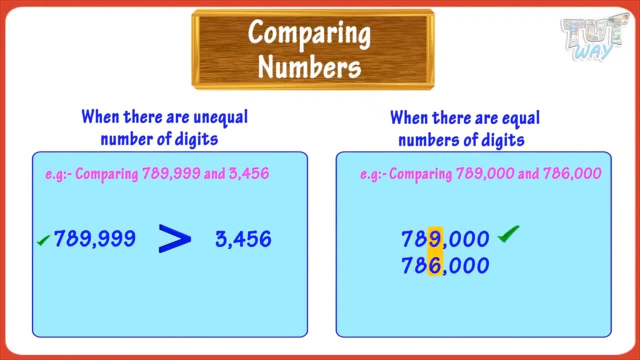 In whichever number we get bigger number first, while comparing each digit, starting from the biggest place, that number is bigger. so 789,000 is more than 786,000.. Let's take another example. We have to compare these numbers and both have same number of digits. Let's start comparing digits from left and in whichever number. 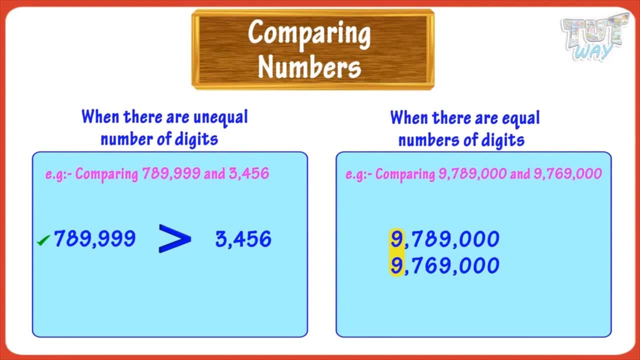 we get the bigger digit first, that number will be bigger than the other one. Comparing the left most digits: both are same. So compare the next digits again. Both are same. Compare the next digit. Here 8 is more than 6. So this number is bigger number. So, kids, let's revise When the 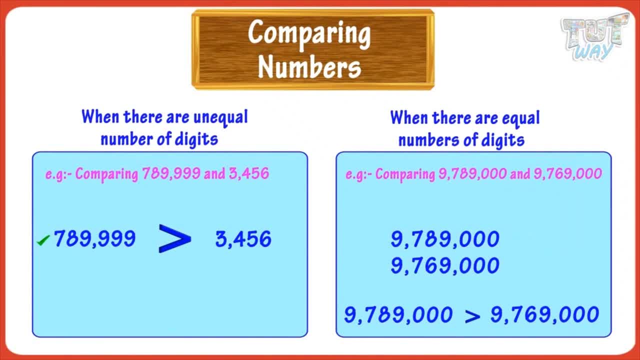 number of digits in two numbers is same. compare the digits to two numbers, starting from the left, and in whichever number you get the bigger number first, that number is the bigger number. So now, kids, now you know how to compare two numbers, no matter how bigger they are. Now let's arrange. 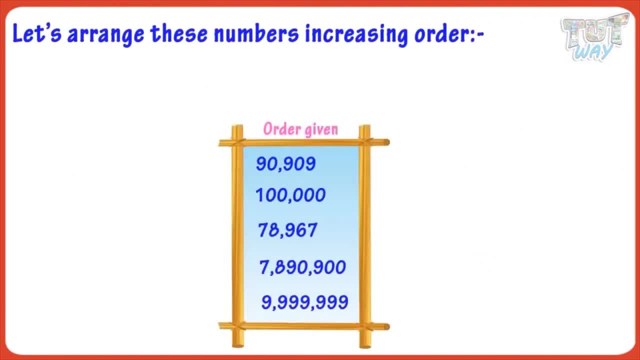 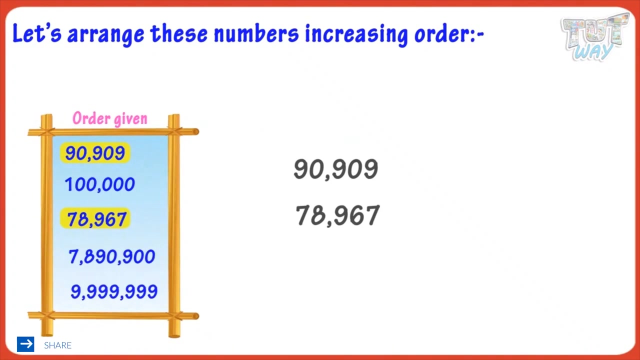 these numbers in increasing order, That is, from smallest to biggest number. Which one is the smallest number here? 78,967 and 90,909 have the least number of digits, so they are the smallest numbers. Now compare them for the smaller number between these. 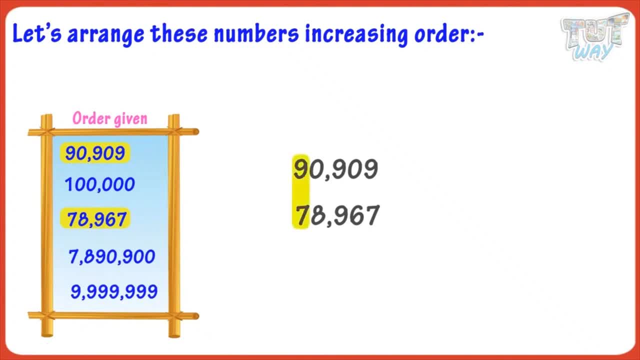 Comparing the first digits, we get: 78,967 is a smaller number, So 8 is more than 6.. So, kids, now you know how to compare two numbers, no matter how big they are. So kids, now you know how to compare two numbers, no matter how big they are. So kids, now you know. 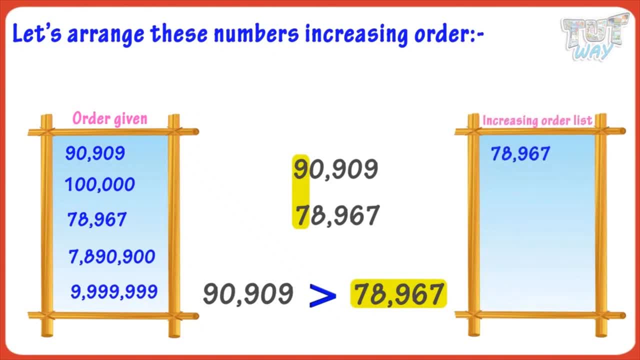 how to compare two numbers, no matter how big they are. So, kids, now you know how to compare two numbers from their first digit. What do you know? Well, 78,967 is smallest, So place it first and cross it from the list. Now, 90,909 is smallest, as it has the least number of digits among the numbers left. 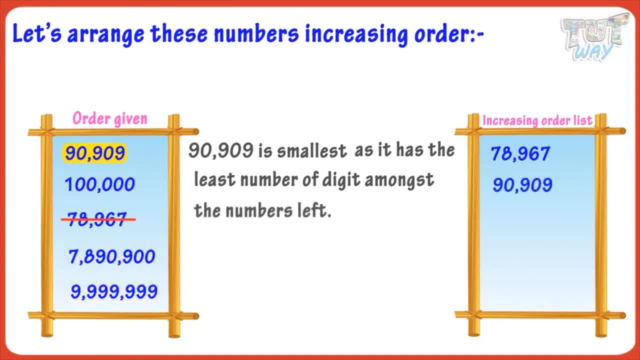 So place it at 2nd place and cross it too from the list. Now. 100,000 has the least number of digits among the numbers left, So place it next and cross it from the list. Now numbers left are same digit numbers, so compare them, Comparing their first digits from: 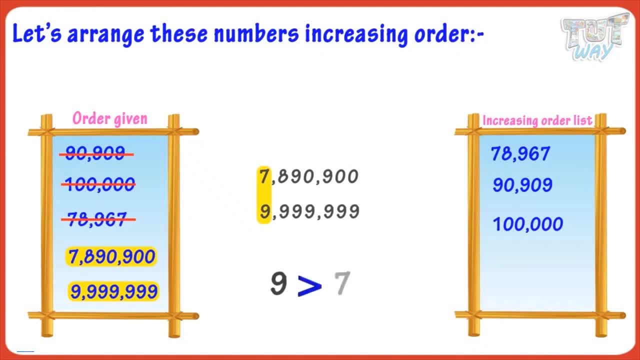 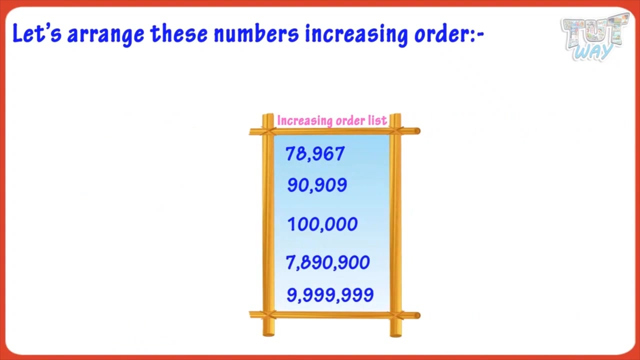 left, that is 9 and 7. We get 9,999,999.. So place it at the last place And place 7,890,900 at the second place, And our increasing order is done. We have arranged the numbers from smallest. 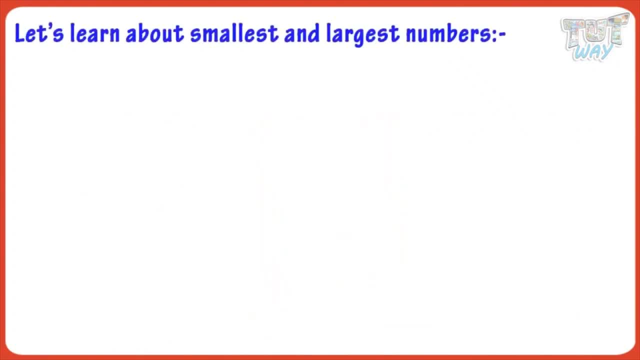 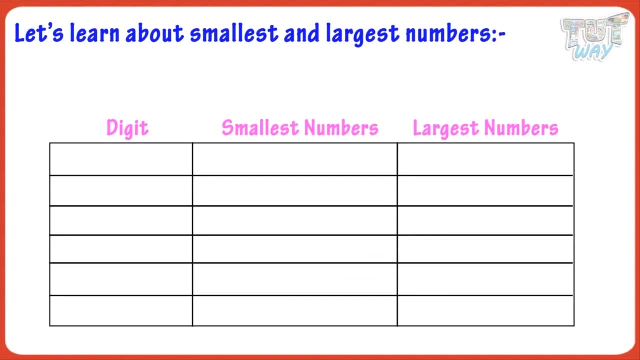 to biggest. Now let's learn about smallest and greatest numbers of particular digits. Kids. here is an interesting pattern of smallest and biggest numbers of particular digits. 1 is the smallest one-digit number. 9 is the largest one-digit number. 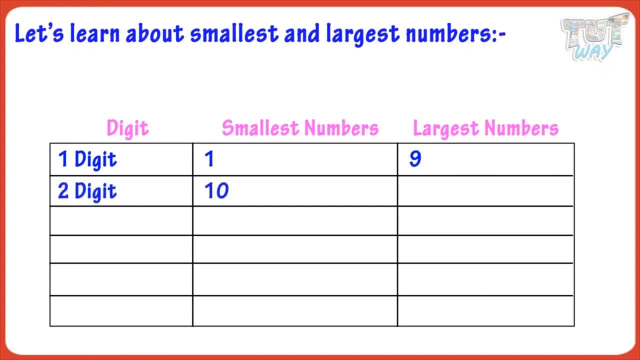 10 is the smallest two-digit number, 99 is the largest one-digit number, 100 is the smallest three-digit number, 999 is the largest three-digit number, 1000 is the smallest four-digit number And 9,999 is the largest four-digit number, And so on. 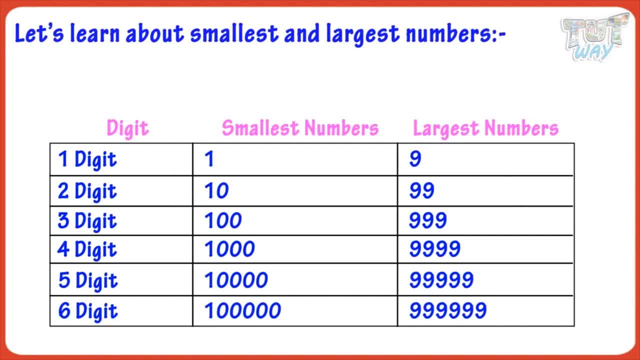 Let's see an interesting thing: If you add 1 to biggest one-digit number, you get the smallest two-digit number. That is, adding 1 to 9, you get 10.. If you add 1 to biggest two-digit number, you get smallest three-digit number. 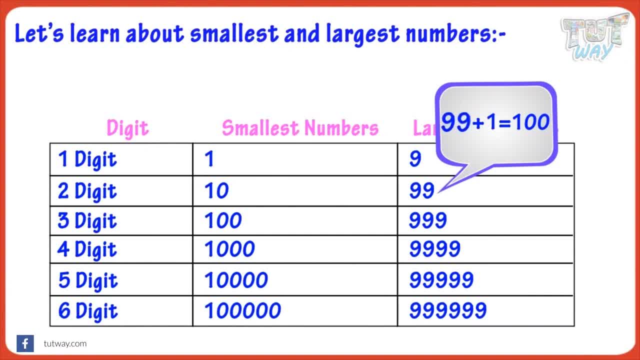 That is adding 1 to 99, you are getting 100.. And if you add 1 to biggest three-digit number, you get smallest four-digit number. That is adding 1 to 999, you will get 1000.. 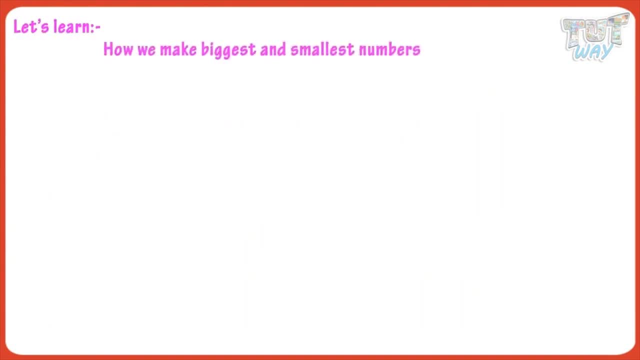 Now we will learn how to make biggest and smallest numbers from the given numbers. Here are four numbers. We have to form the largest four-digit number using these numbers only. Also, we do not have to repeat any number. Okay, kids, let me help you. do that. We have to make a four-digit number. We need to have the